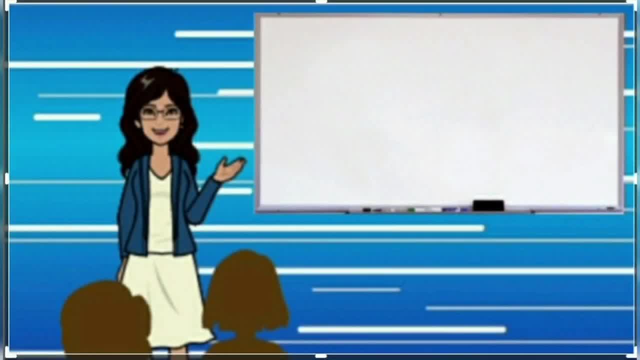 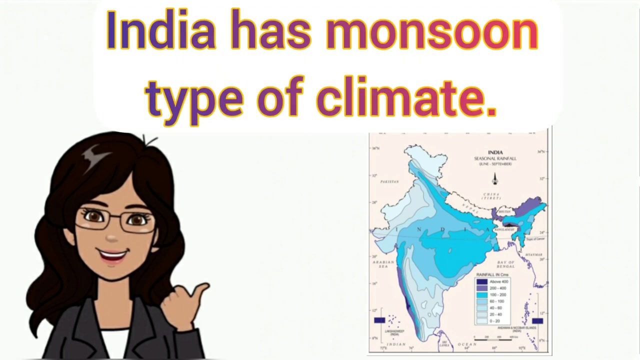 you can experience different weather, Whereas climate is defined as the average weather condition of a place for a longer period of time, ie more than 30 years, And it is always of a large area, for example India. In India, we have a monsoon type of climate. Do you know why this name has been? 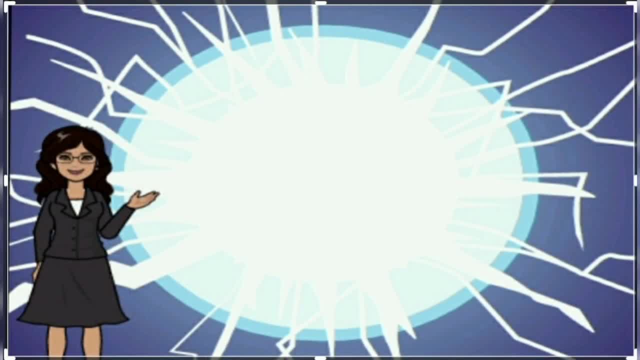 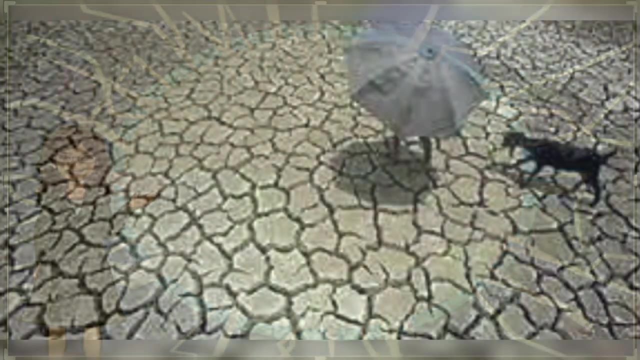 given to India's climate. It is because of the monsoon climate In India, the monsoon winds that blow in our country and bring most of the rainfall, in which season Monsoon season. By now you must have understood that the weather can change. 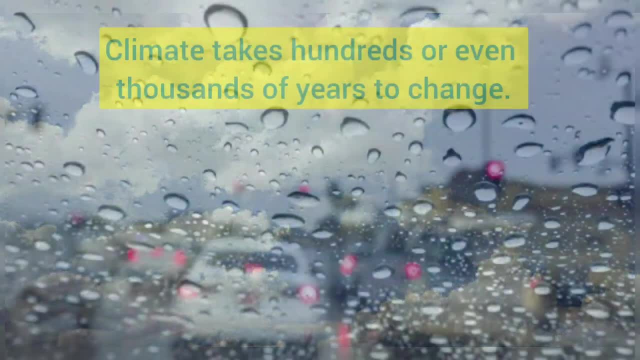 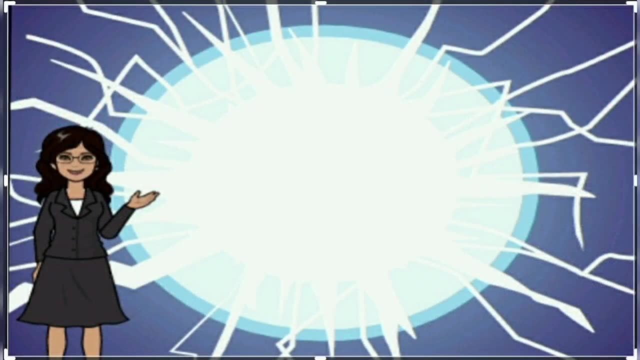 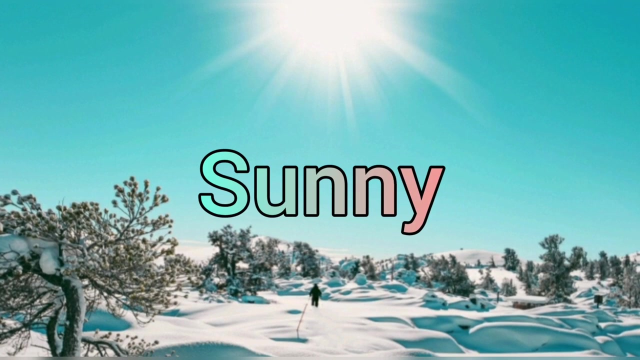 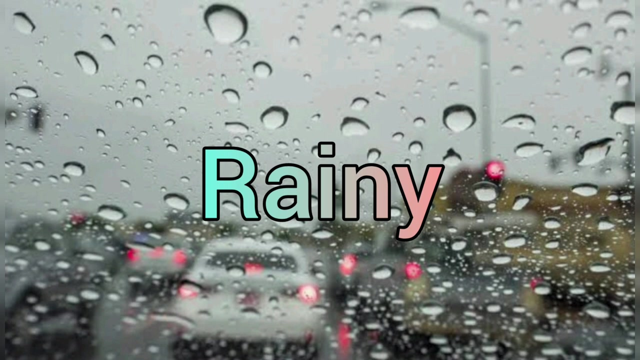 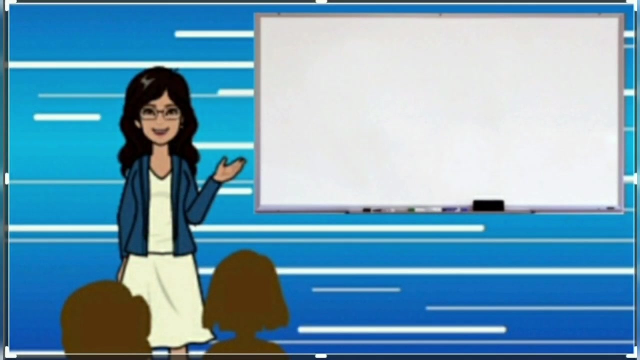 in just a few hours, Whereas climate takes hundreds or even thousands of years to change. Everyday, we use a variety of terms such as hot, cold and cold. These terms are used to describe weather conditions. Actually, these terms explain the atmospheric conditions with respect to air temperature. 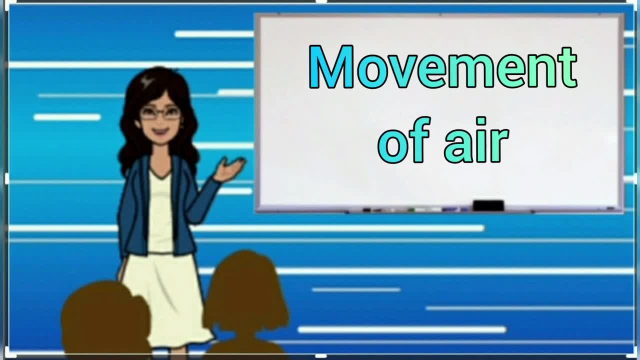 air pressure, movement of air, humidity, etc. We will see the following terms in the next class. These are the main elements of a weather context: 5. Air temperature, Air pressure, Movement of air, Humidity, etc. These are the main elements of a weather context. 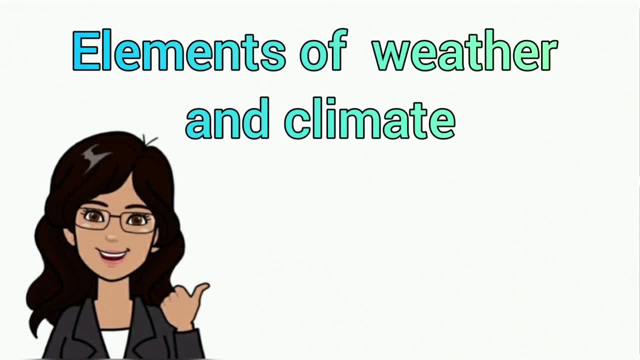 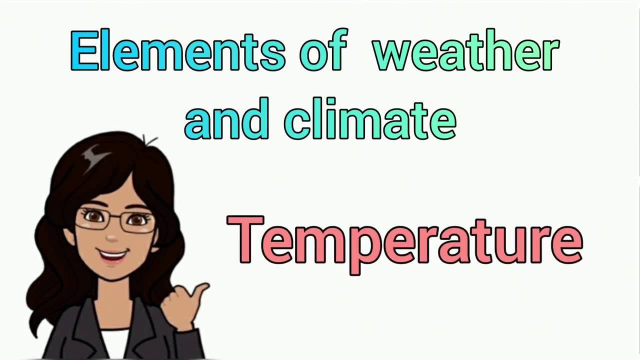 1.Modulation from a weather context. 2.Air pressure, Air used on air or cooling or heating or cooling air. air infiltration, wind of weather and climate. Let us know about each element in detail. The first one is Temperature. 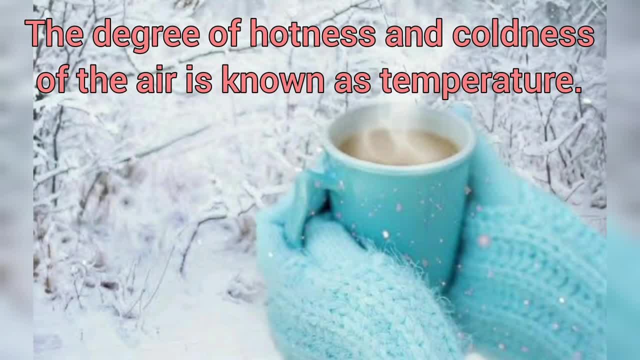 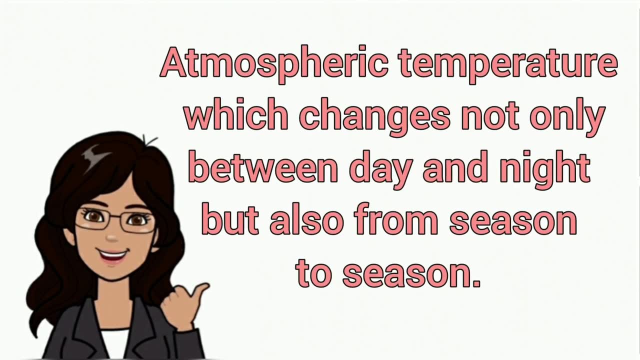 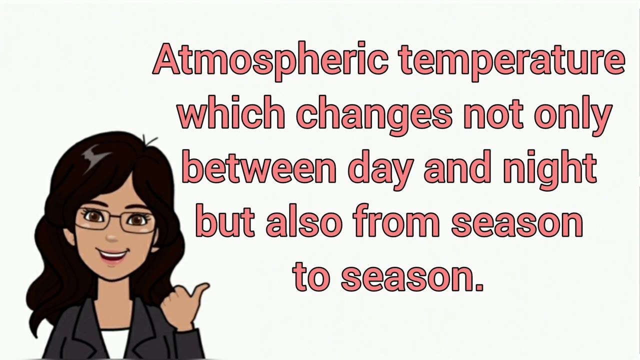 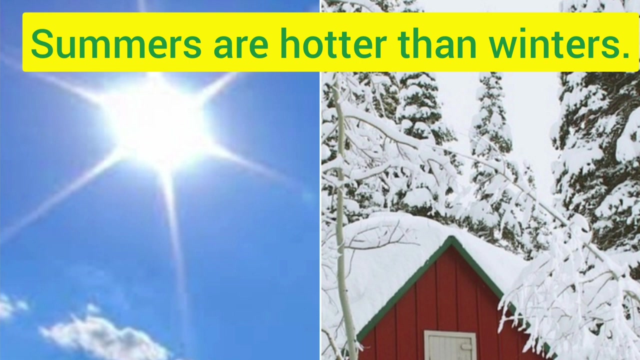 The degree of hotness and coldness of the air is known as temperature. Here we will talk about the atmospheric temperature, which changes not only between day and night, but also from season to season. For example, summers are hotter than winters. These differences in temperature exist because the amount of solar radiation received on 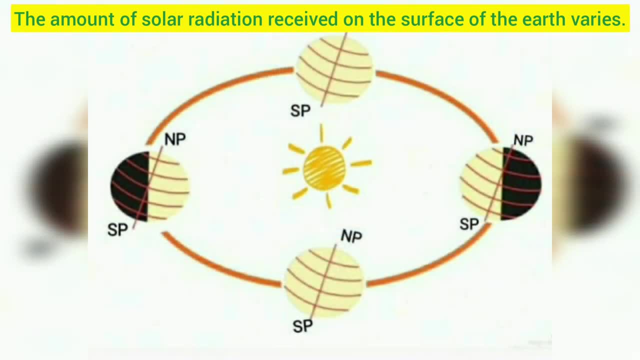 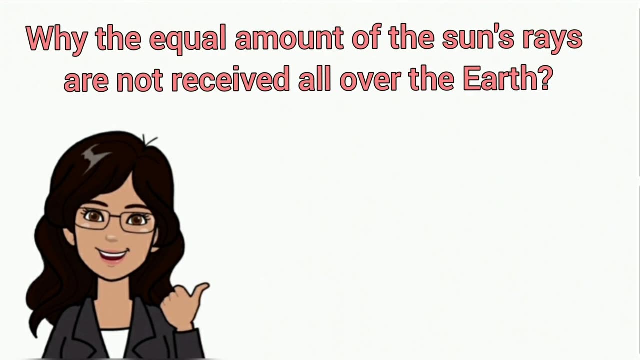 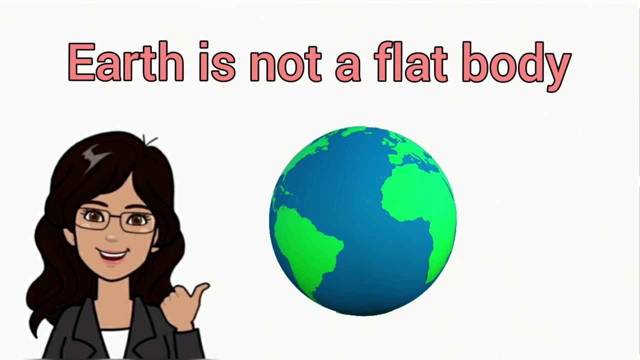 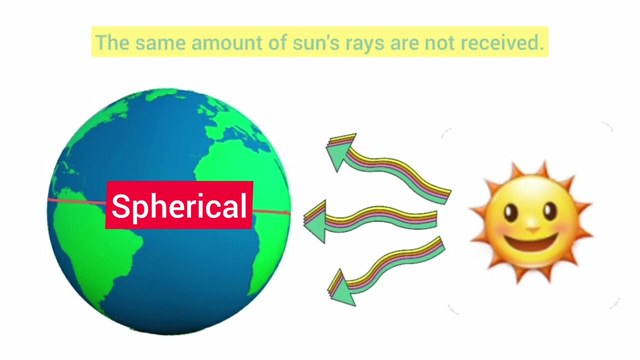 the surface of the earth varies from place to place and from time to time. Now you can ask a question: why the equal amount of sun's rays are not received all over the earth? Because our earth is not a flat planet. It is almost spherical in shape, due to which the same amount of sun's rays are not received. 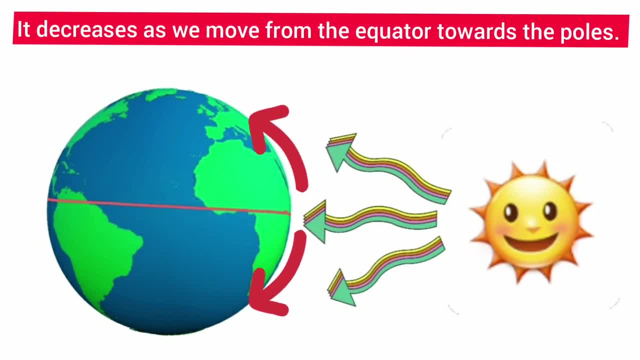 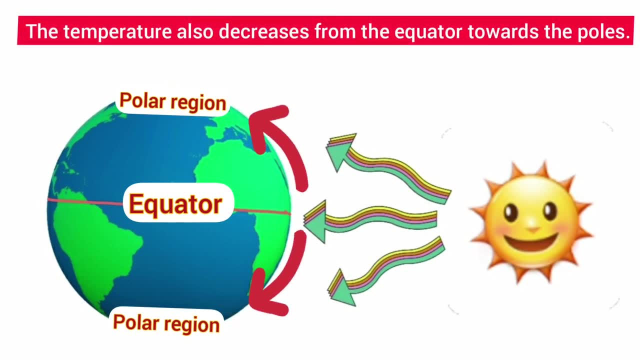 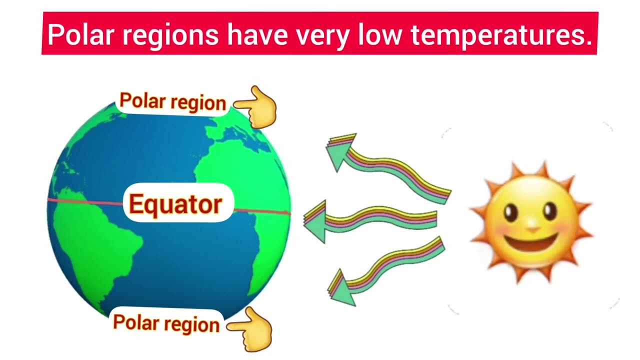 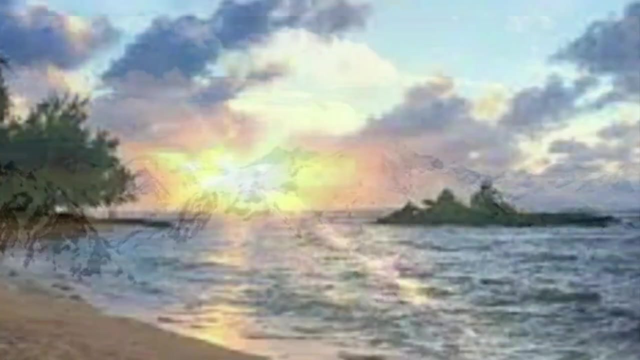 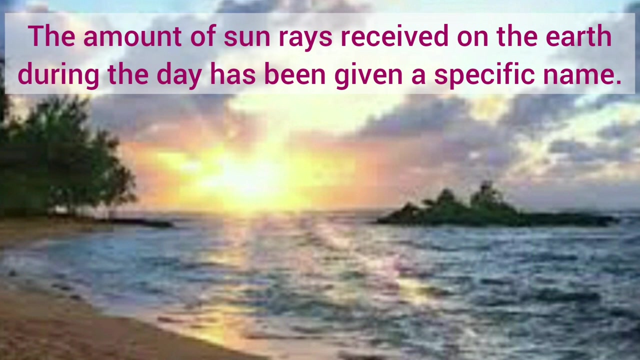 everywhere. It decreases as we move from equator towards the poles. As a result, the temperature also decreases from equator towards the poles. Hence the polar regions have very low temperature. The amount of solar radiation received on the earth during the day has been given a. 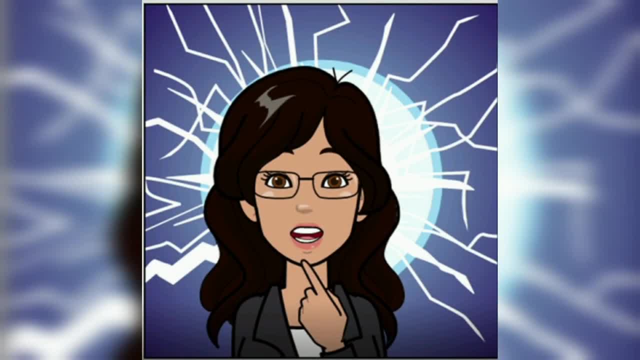 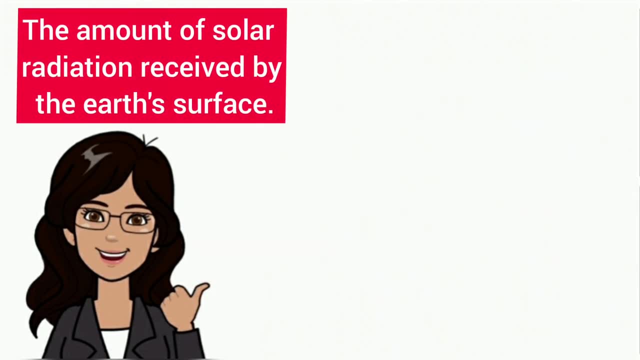 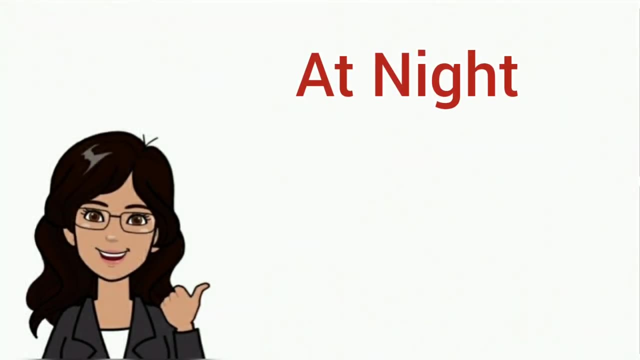 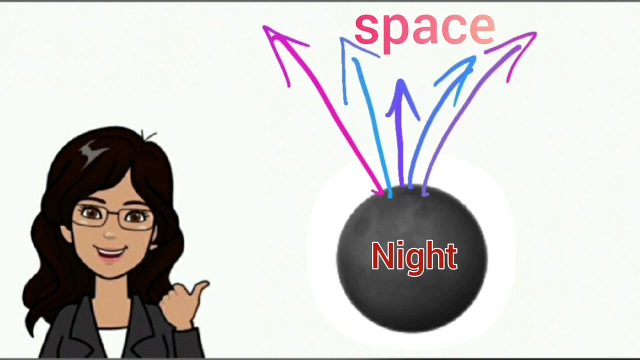 specific name. Any ideas? what do we call it? It is called Insulation, So insulation can be defined as the amount of solar radiation received by the earth's surface during the day. At night, The heat which was absorbed during the day is radiated back to space. 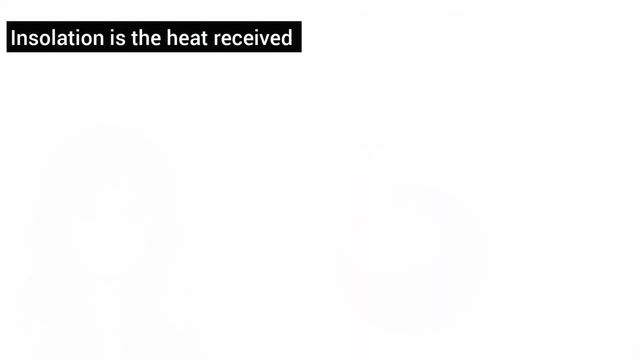 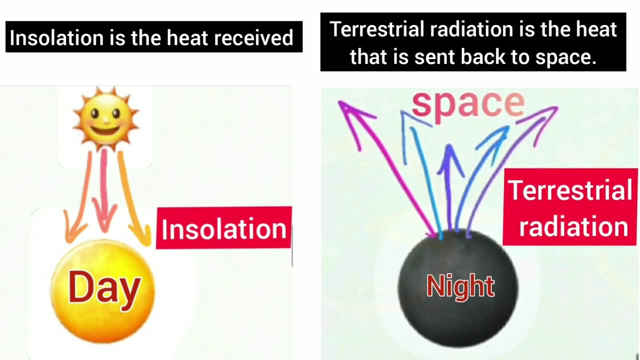 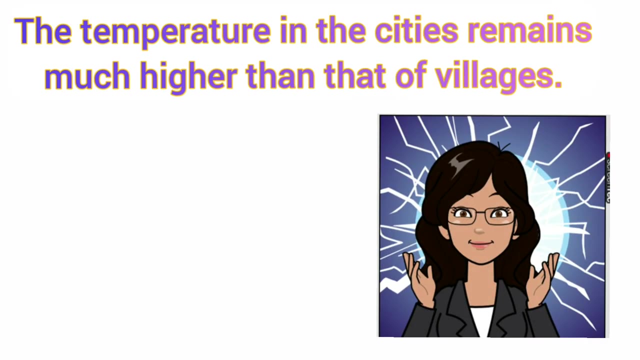 This is called terrestrial radiation. So insulation is the heat received and terrestrial radiation is the heat that is sent back to space. Now I have a question for you. You must have heard that the temperature in the cities remains higher than that of the villages. 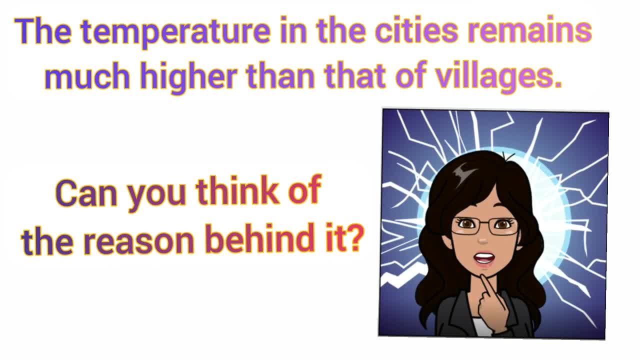 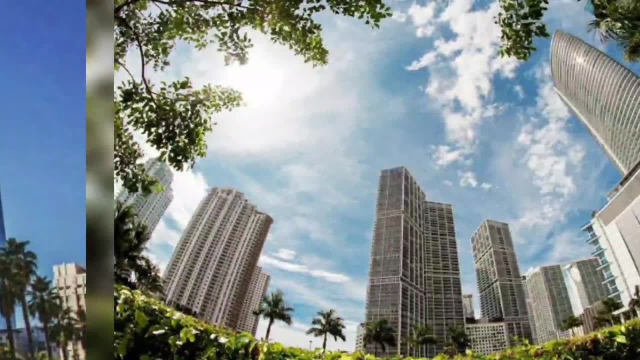 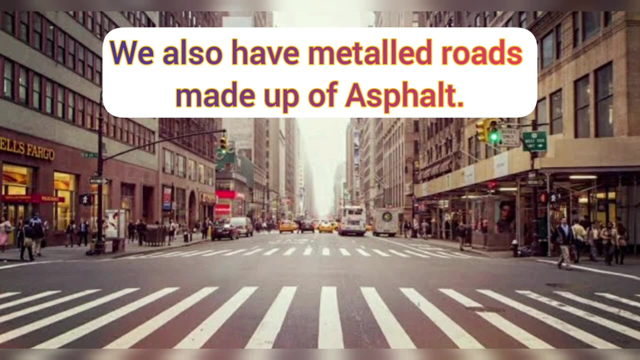 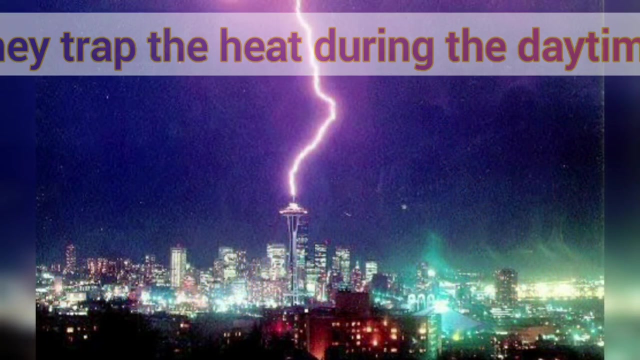 Can you think of the reason behind it? Let me tell you, You know, we have high rise buildings in cities that are made up of concrete and metals, And we also have metal roads made up of asphalt. They trap the heat during the daytime and release it during the night. 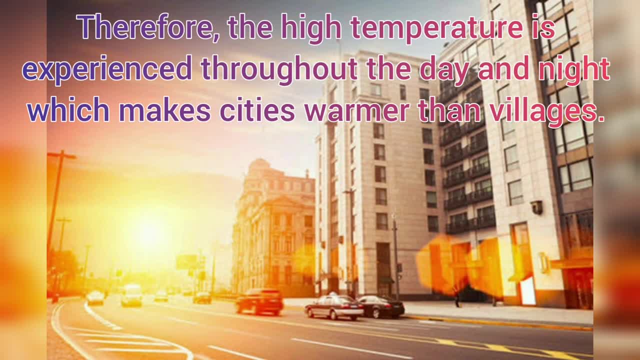 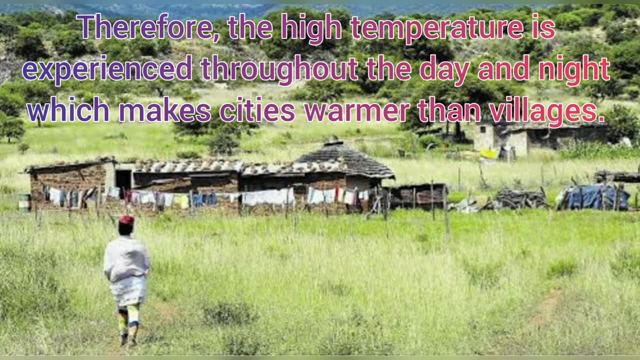 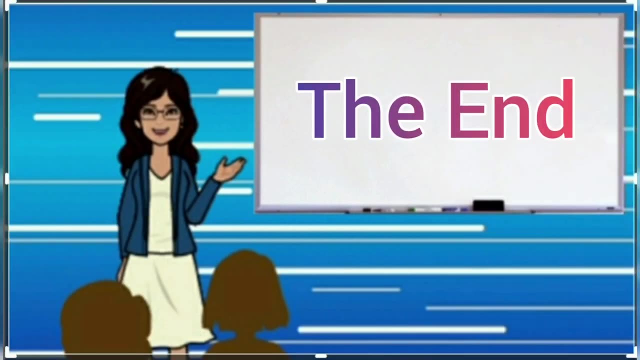 Therefore, The high temperature is experienced throughout the day and night, Which makes cities warmer than villages. Hope you understood the reason why cities are warmer than villages. So, children, let us end today's class here. In the next video we will continue with air pressure.